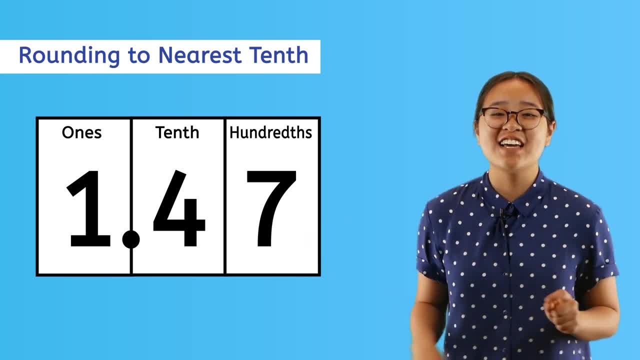 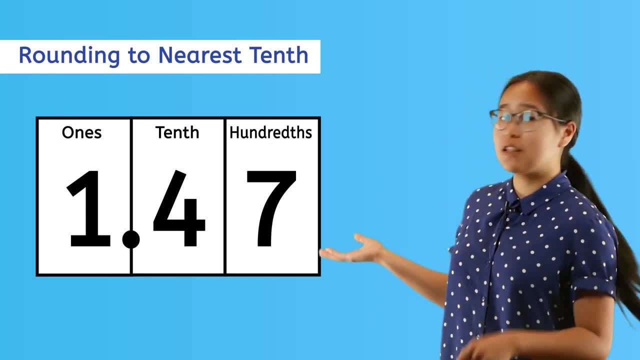 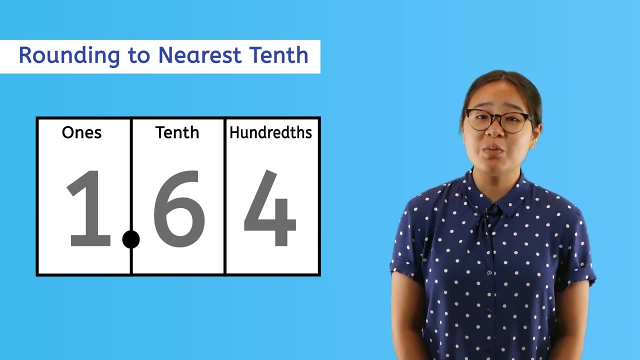 Our first number is 1.47.. The digit in the hundredths place is 7, so we round up This number. rounded to the nearest tenth is 1.5.. 1.64 has a 4 in the hundredths place. 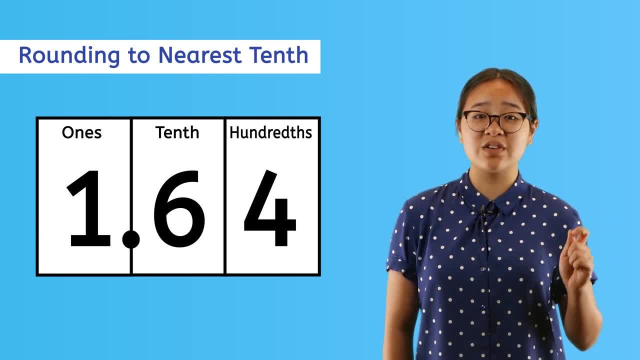 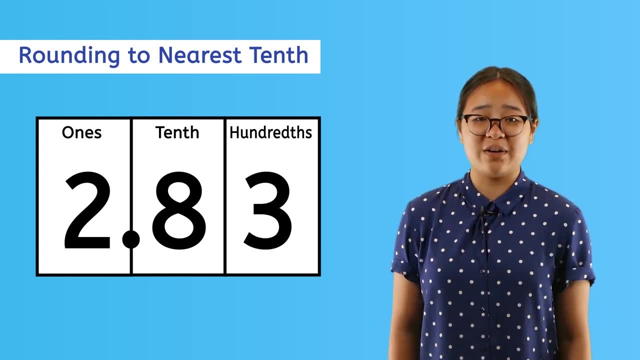 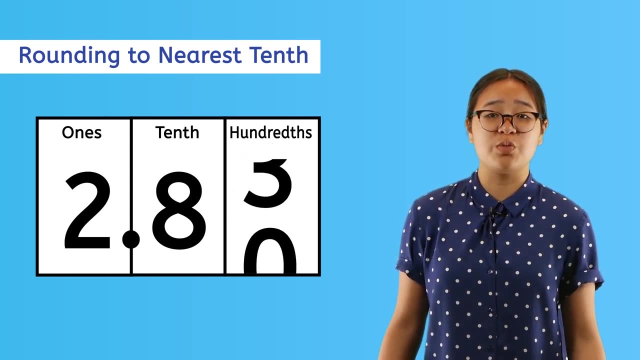 4 rounds down, so this is 1.6.. 2.83 also rounds down, since there is a 3 in the hundredths place, So it becomes 2.8.. Finally, 4.97 rounds up. 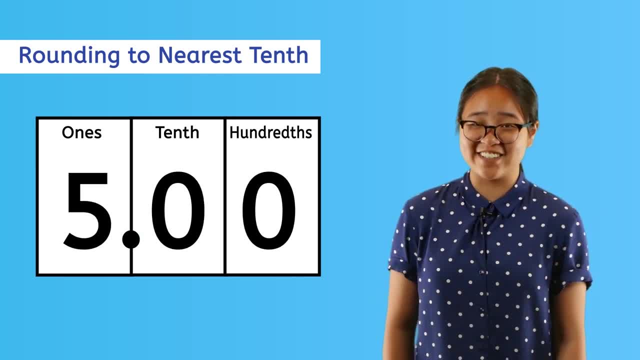 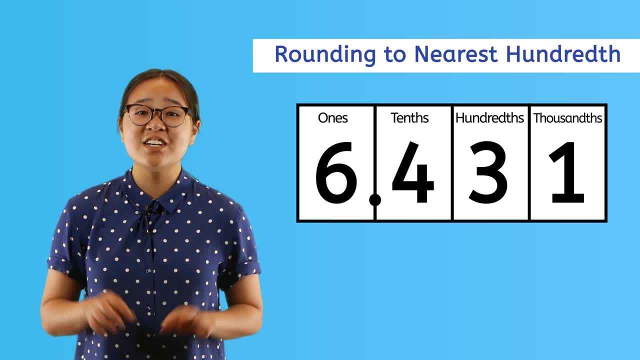 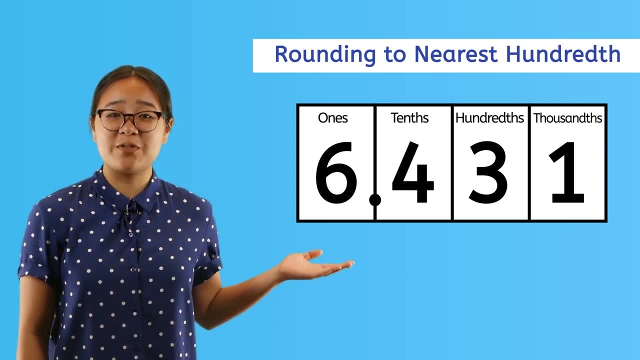 If we round up, this becomes 5.0.. If you have a long decimal number with numbers in the thousandths place, you'll look at the digit in the thousandths place to see how to round 6.431 rounds down to 6.43.. 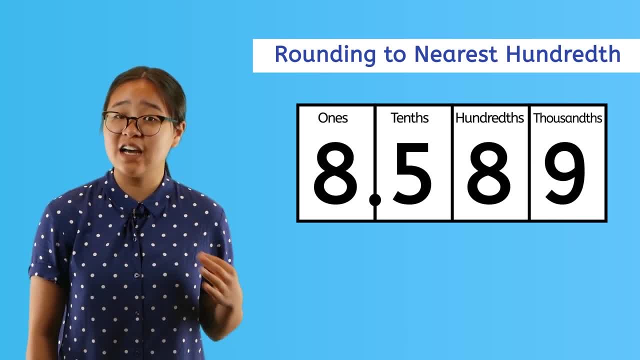 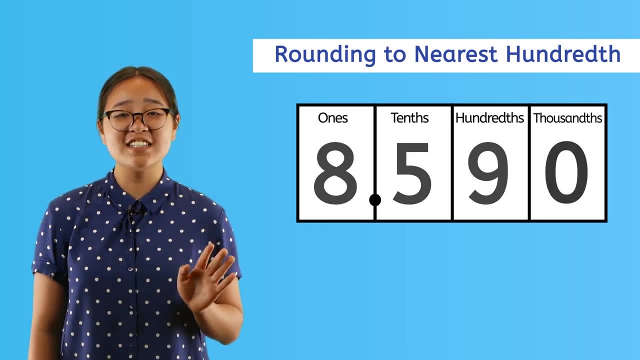 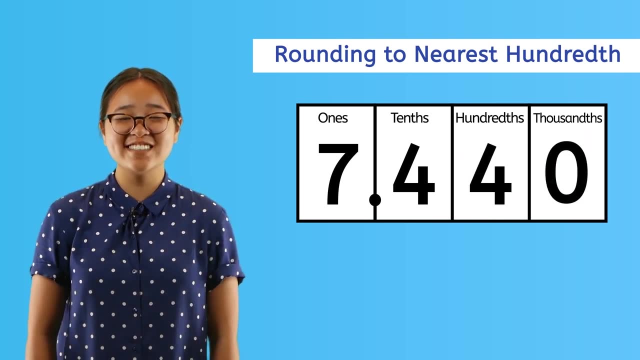 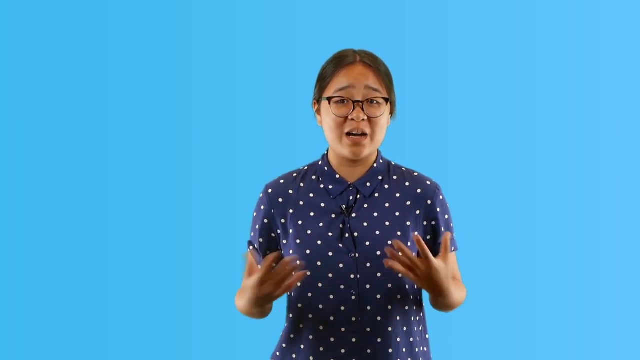 8.589 rounds up to 8.59.. And 7.438 rounds up to 7.44.. Now you know how to round decimals to the hundredth or tenth place, but you still need to learn how to round them to the nearest whole number. 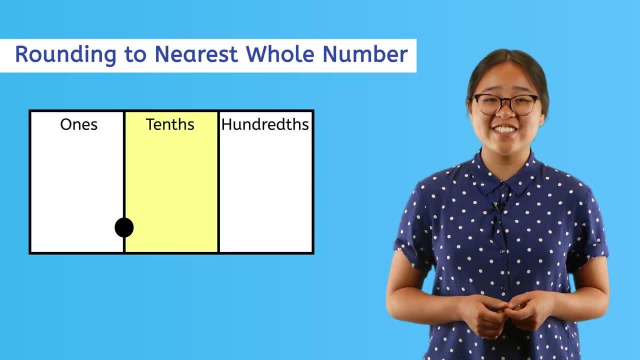 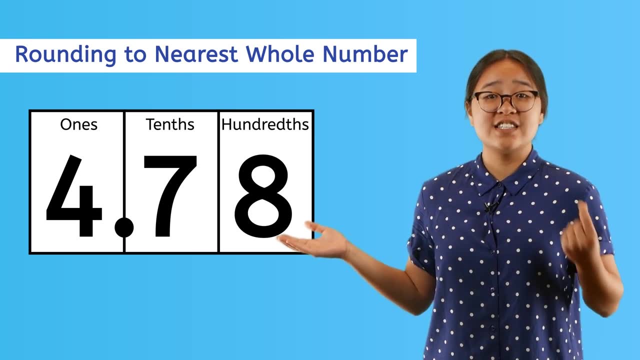 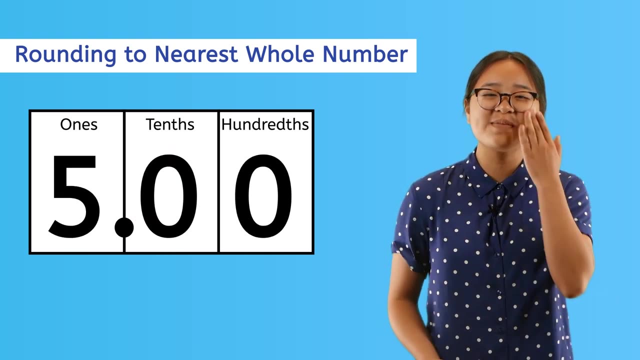 You'll look at the tenth place to know which way to round The number 4.78, rounds up to 5, since 7 is more than 5, and numbers greater than 5 round up. 6.24 rounds down. 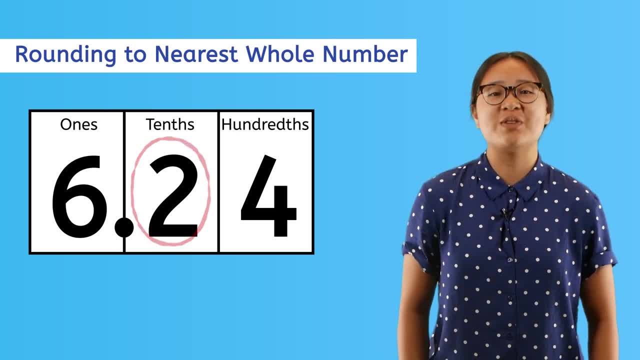 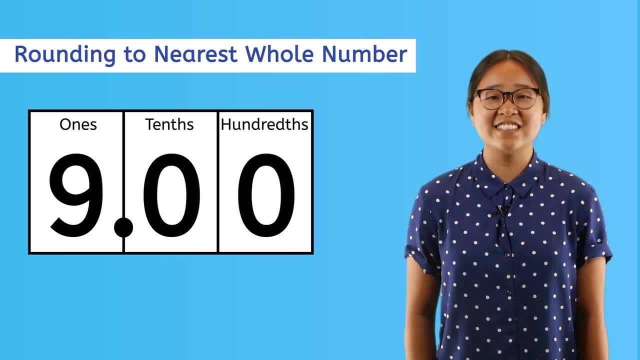 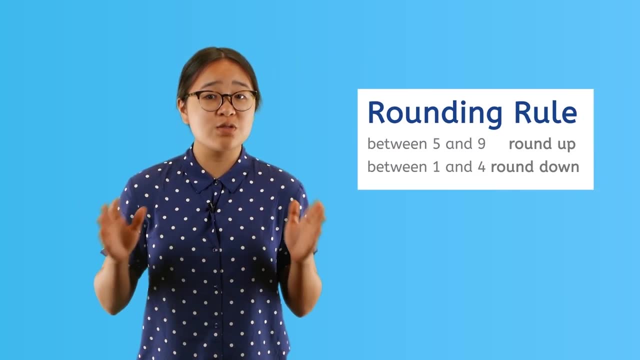 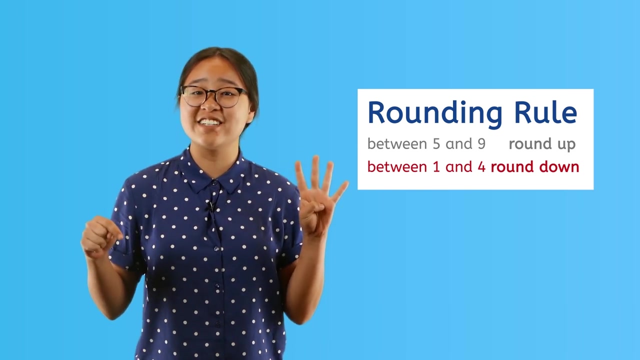 because numbers 4 or lower round down. 9.47 rounds down to 9.. The rules of rounding are the same for decimals as they are for other numbers. If you can remember, those rules round up for 5 or over and down for 4 or under. 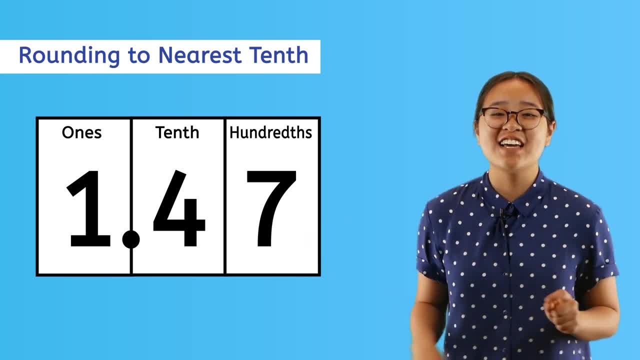 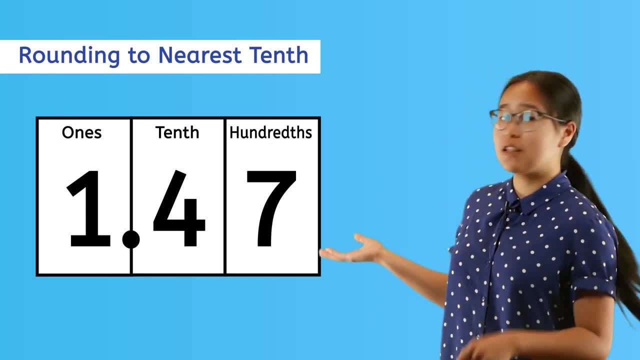 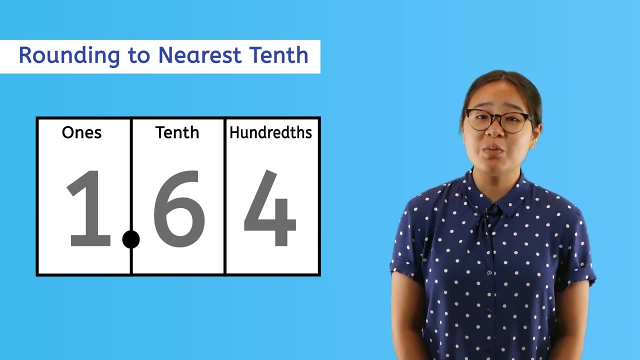 Our first number is 1.47.. The digit in the hundredths place is 7, so we round up This number. rounded to the nearest tenth is 1.5.. 1.64 has a 4 in the hundredths place. 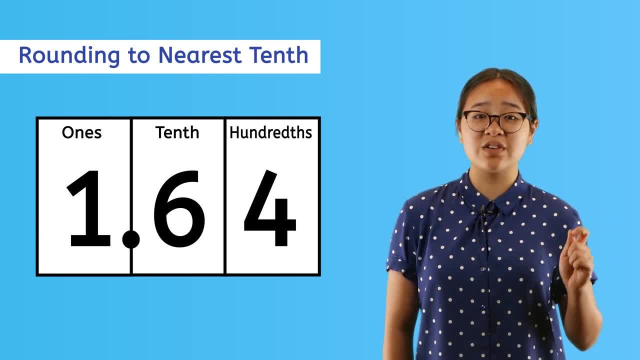 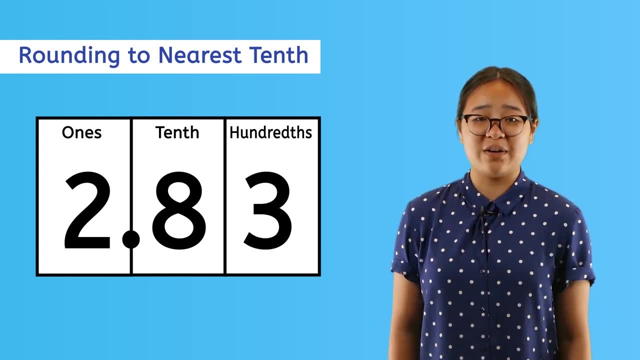 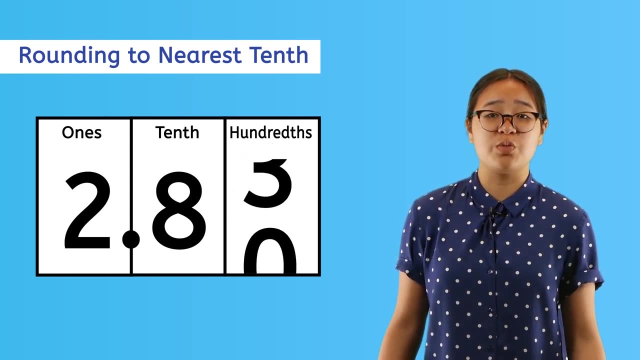 4 rounds down, so this is 1.6.. 2.83 also rounds down, since there is a 3 in the hundredths place, So it becomes 2.8.. Finally, 4.97 rounds up. 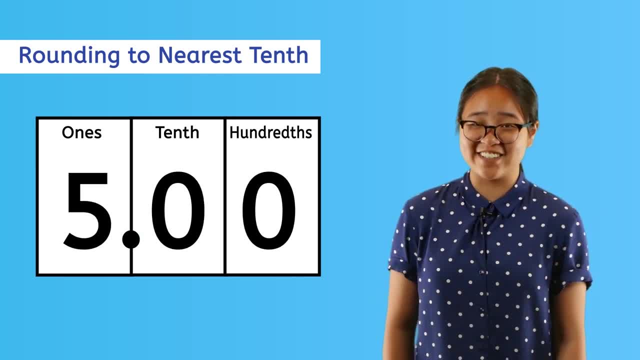 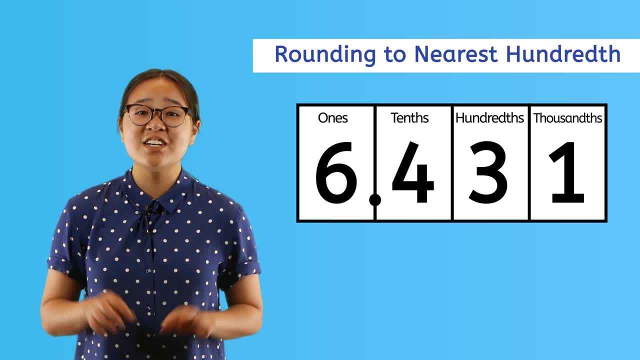 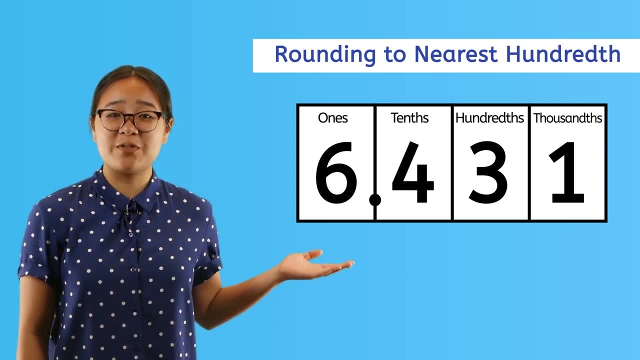 If we round up, this becomes 5.0.. If you have a long decimal number with numbers in the thousandths place, you'll look at the digit in the thousandths place to see how to round 6.431 rounds down to 6.43.. 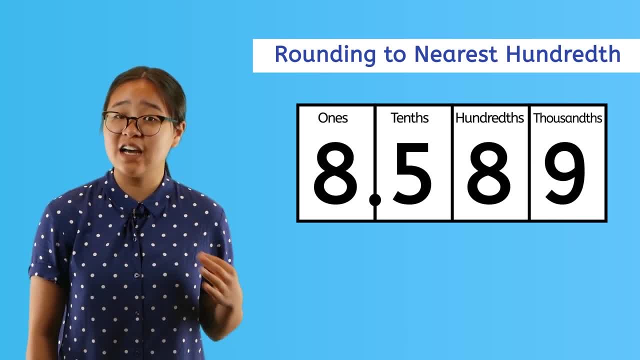 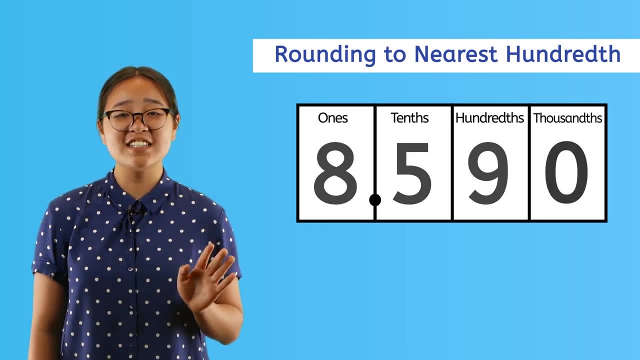 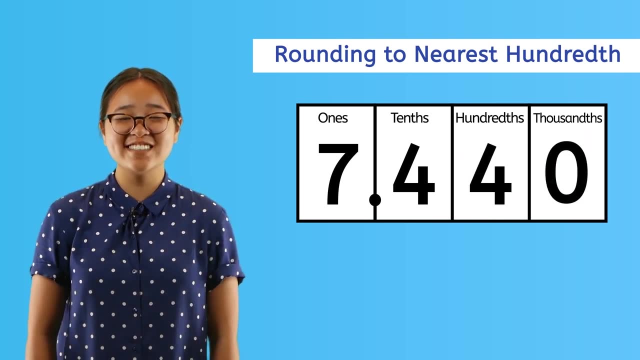 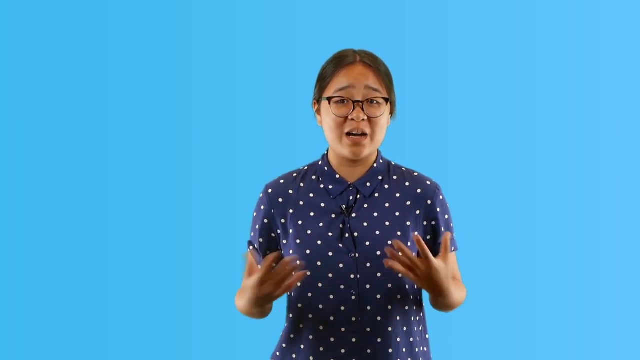 8.589 rounds up to 8.59.. And 7.438 rounds up to 7.44.. Now you know how to round decimals to the hundredth or tenth place, but you still need to learn how to round them to the nearest whole number. 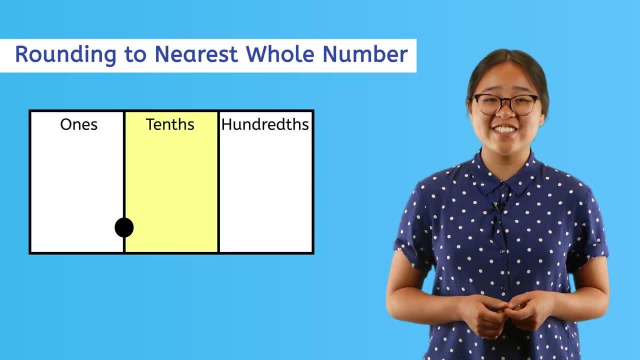 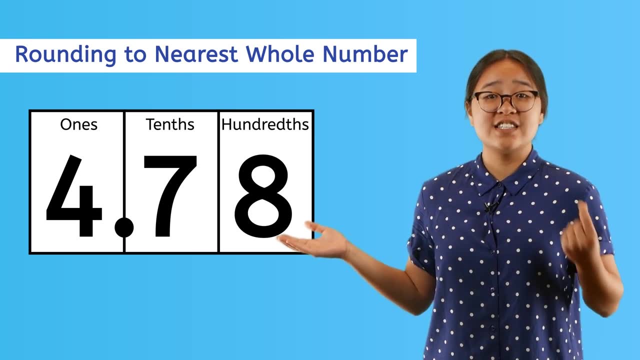 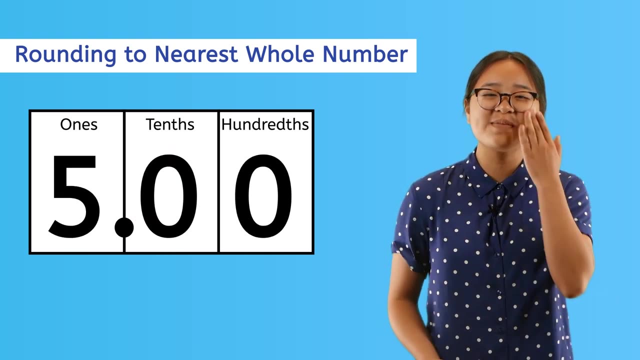 You'll look at the tenth place to know which way to round The number. 4.78 rounds up to 5,. since 7 is more than 5, and numbers greater than 5 round up 6.24 rounds down. 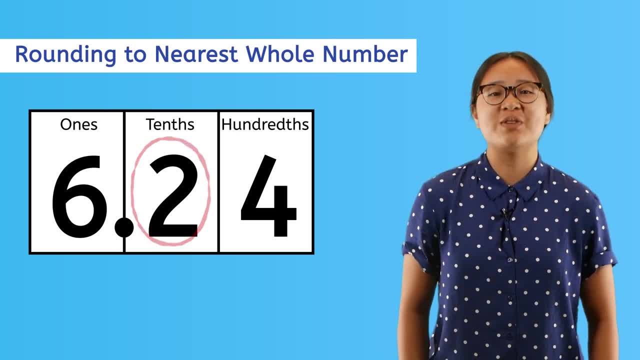 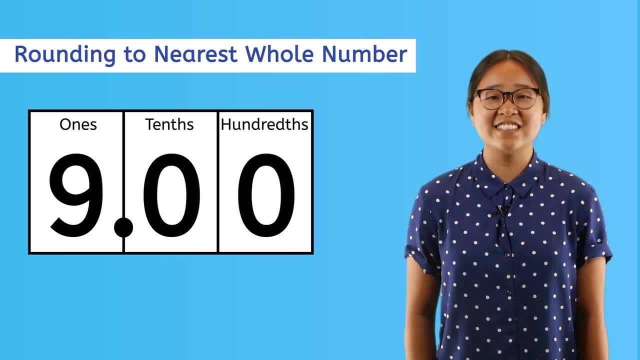 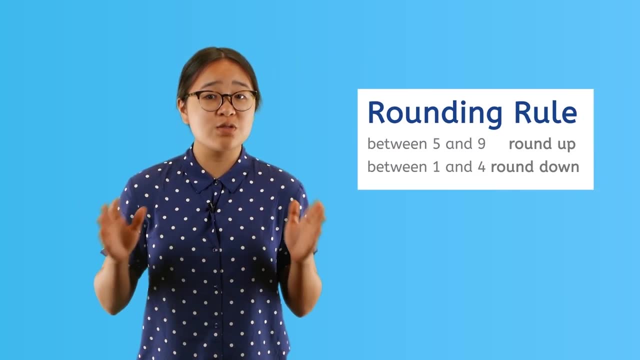 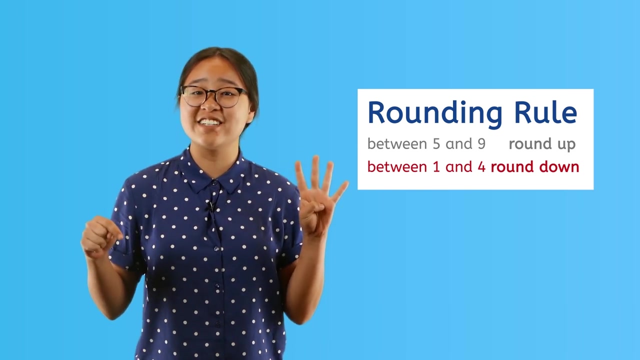 because numbers 4 or lower round down. 9.47 rounds down to 9.. The rules of rounding are the same for decimals as they are for other numbers. If you can remember, those rules round up for 5 or over and down for 4 or under. 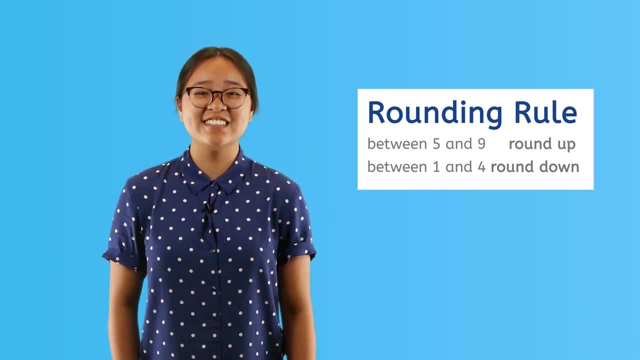 you can round decimals just like you do whole numbers. Keep your rounding rules in mind and remember always be clever.